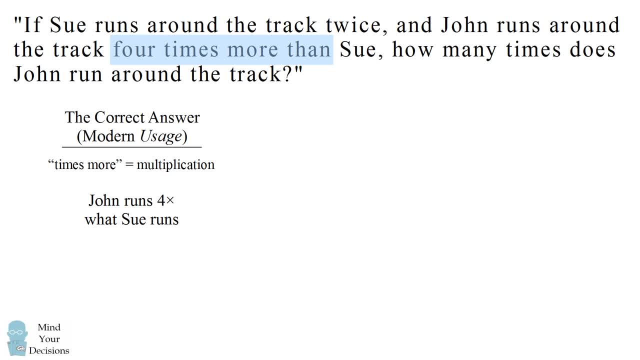 that Sue runs. So we take four times two to get to the answer of eight. Other people had a different interpretation of this problem. They read this as saying: John runs around four times more as an addition. So if Sue runs around the track two times, John runs four more laps than Sue. This is. 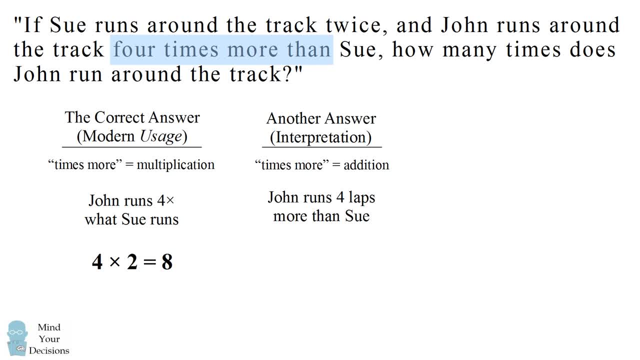 four more times. So the number of times that John would run would be four plus two, which equals six. The problem with this interpretation is we usually write more times when we're referring to addition and when we have the phrase times more, we're usually referring to multiplication. 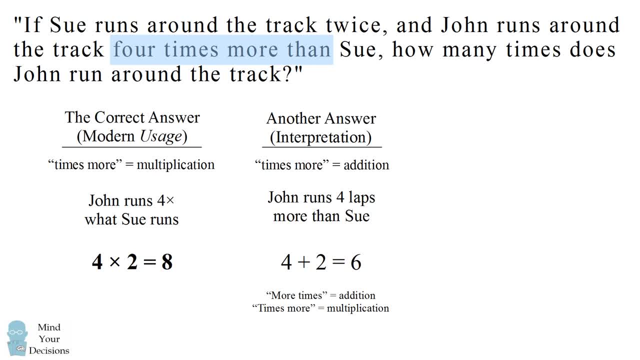 There's a third way to read this problem which would be literally correct according to these words. on a strict grammatical basis, The literal version of this problem is often used in terms of percentages. Times more than would mean you should add that number of times to the base, So think. 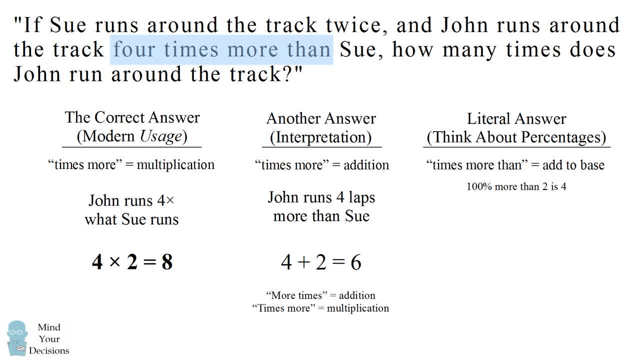 about this in terms of percentages, 100% more than 2 is a total of 4,. 200% more than 2 is a total of 6,, 300% more than 2 is a total of 8, and 400% more than 2 is a total of 10.. So 400% more is. 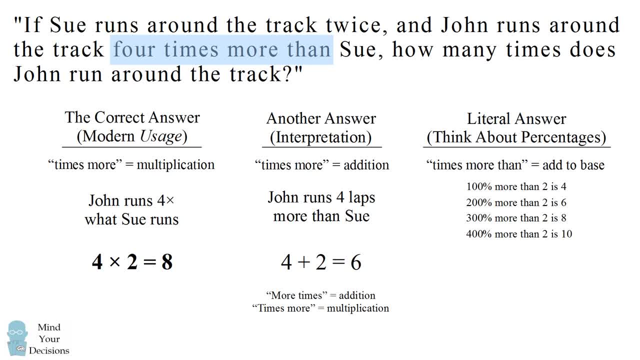 the same thing as 4 times. so having 4 times more than Sue would mean 4 times 2 plus 2, which would equal 10 times. So this is an interpretation that's literally correct, according to the way the sentence is written, However, in